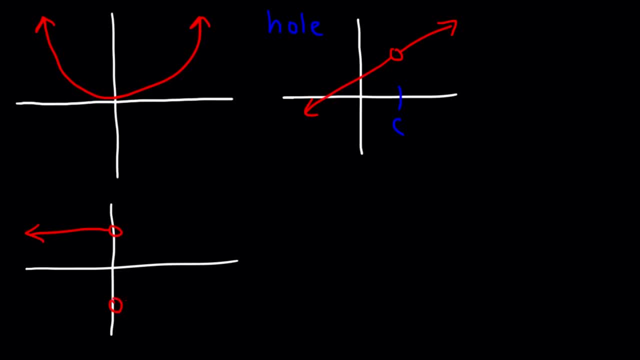 Here's another type of discontinuity, and this one is called a jump discontinuity, because the left side and the right side do not connect. And then there's another type. This type of discontinuity is known as an infinite discontinuity. As you approach the vertical asymptote on the right side, it approaches positive infinity. 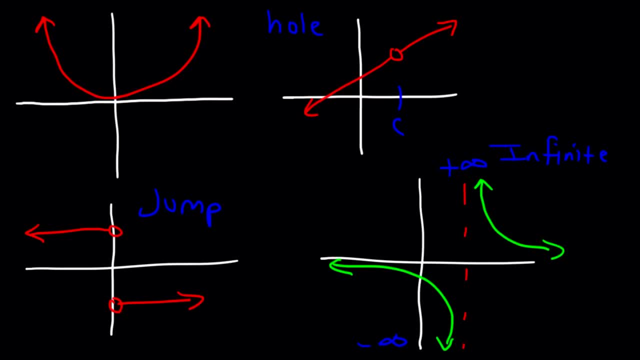 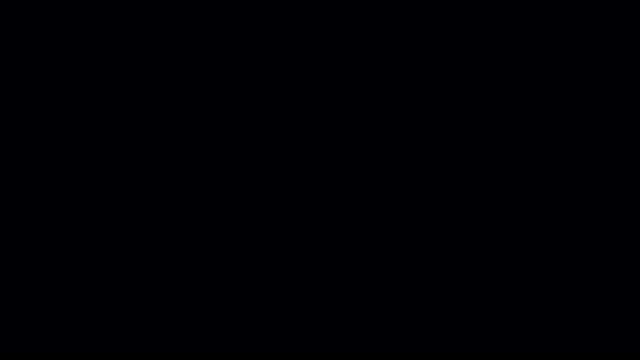 on the left, negative infinity. Now you need to know that the whole is a removable discontinuity. But the other two, the jump discontinuity and the infinite discontinuity, are non-removable discontinuities. Now let's talk about how to identify points of discontinuity in 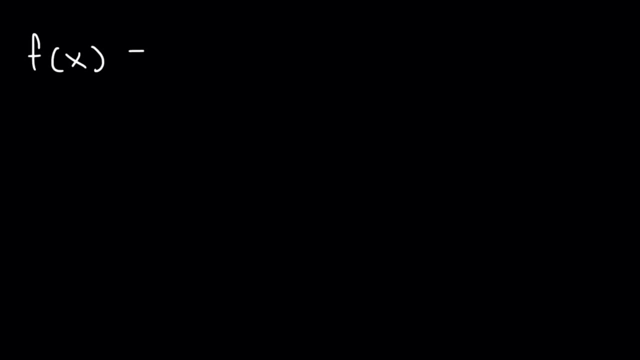 the graph. We're going to talk about how to identify points of discontinuity in the graph. So here's the first example: 1 over x squared. If you're given a rational function, you could find the vertical asymptote, which is an infinite discontinuity. 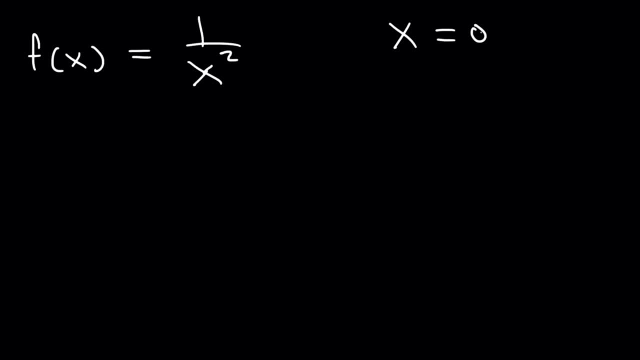 by setting the denominator equal to 0. So in this case the vertical asymptote is: x equals 0. So therefore, that's a point of discontinuity, because in this graph there is no x value of 0. It's undefined at that point And, as you can see, we have 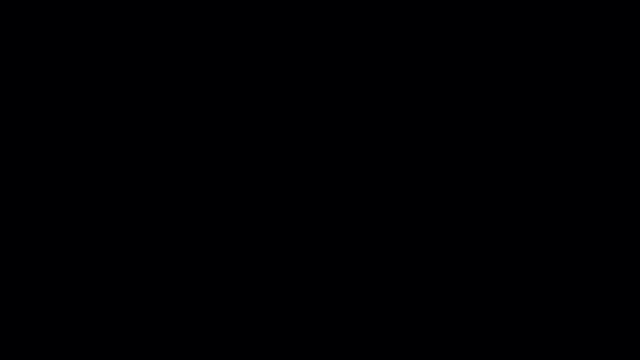 an infinite discontinuity. So here's another example. Let's say if we have 5 divided by x plus 2.. x plus 2 cannot be 0 because that's going to be the vertical asymptote. So therefore x cannot be negative 2.. That is the point of discontinuity. 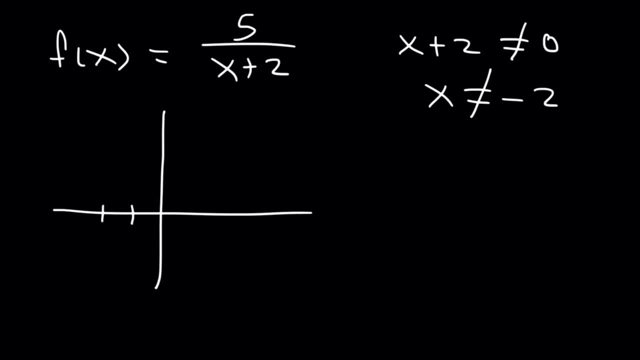 If we graph this function, we're going to have a vertical asymptote at: x equals negative 2. And so the graph is going to look something like this: So this is another infinite discontinuity. Now what about a function that looks like this, Let's say, 3 times x plus 2,. 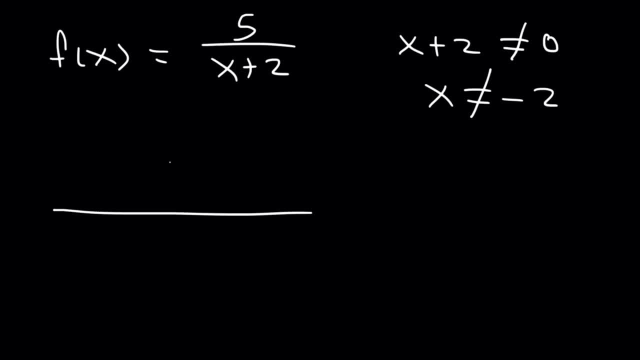 x cannot be negative two. That is the point of discontinuity. If we graph this function, we're going to have a vertical asymptote at x equals negative two, And so the graph is going to look something like this: So this is another infinite discontinuity. 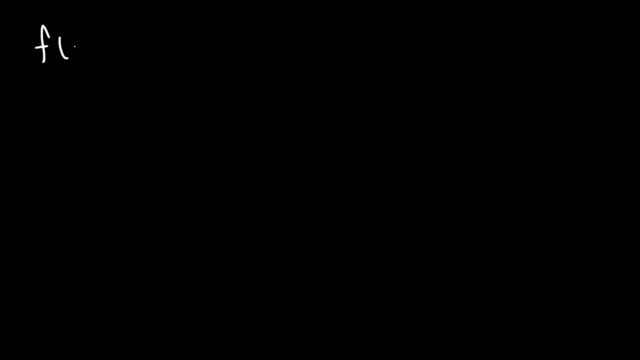 Now what about a function that looks like this. Let's say three times x plus two divided by x plus two times x minus five, The x minus five factor on the bottom leads to the vertical asymptote. So x cannot equal zero. So that is an infinite discontinuity Anytime it's associated with a vertical asymptote. 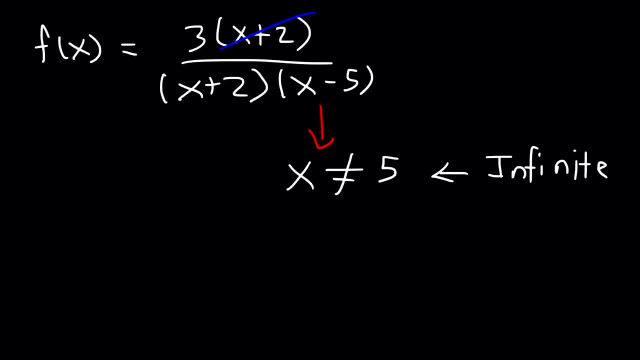 it's an infinite discontinuity. Now notice that we can cancel x plus two. However, this is still a point of discontinuity. So x cannot equal negative two, But this type of discontinuity is known as a whole, if it can be canceled. Here's another problem. 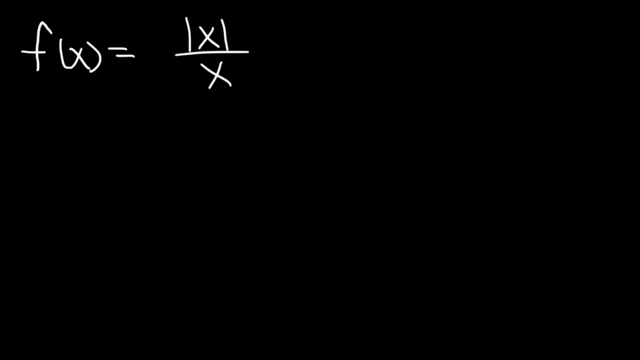 x is equal to the absolute value of x divided by x. So what type of discontinuity do we have in this example? Is it a whole, a jump discontinuity or an infinite discontinuity? Also determine if it's removable or non-removable. 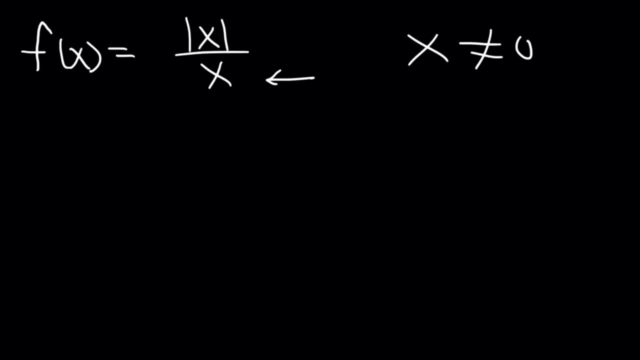 Now we know that the denominator can be zero, So x cannot equal zero. But notice that we have an absolute value function. So this could be positive x, which means f of x can be one, or negative x, which means f of x can be equal to negative one. 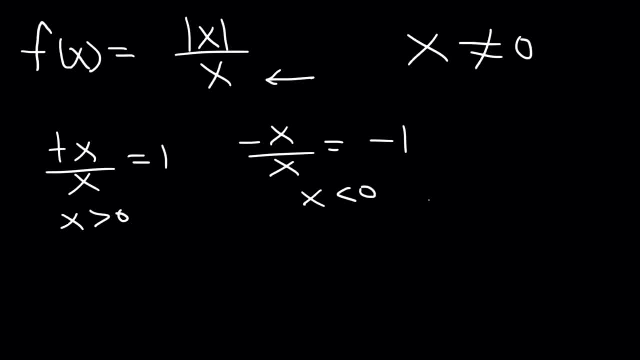 This is true when x is greater than zero, and this is true when x is less than zero. So the graph looks something like this: When x is greater than one and 0,, it is going to be positive one and when it is less than zero, negative one. 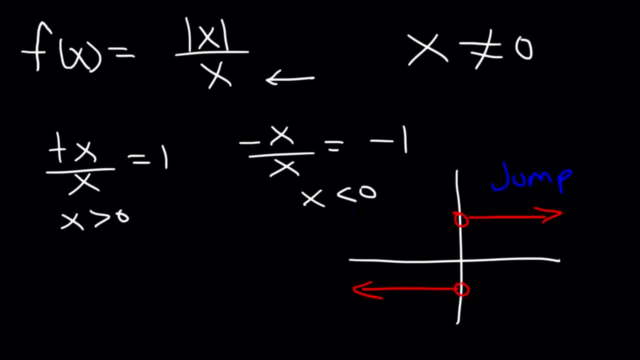 So this is the jump discontinuity, And it usually occurs whenever you have an absolute value function like this, or It could be due to a piecewise function as well. Now, a jump discontinuity is also a non-removable discontinuity. 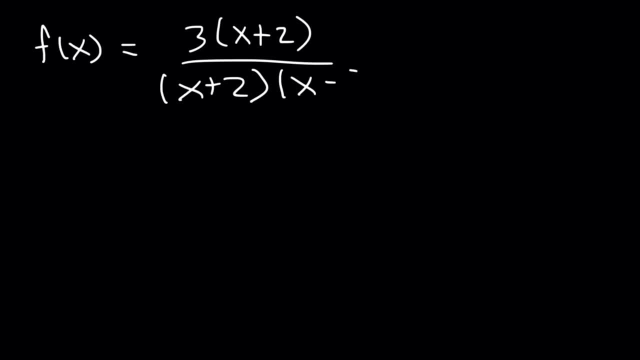 divided by x plus 2 times x minus 5. The x minus 5 factor on the bottom leads to the vertical asymptote. so x cannot equal 0. positive 5.. So that is an infinite discontinuity Anytime it's associated with a vertical asymptote. 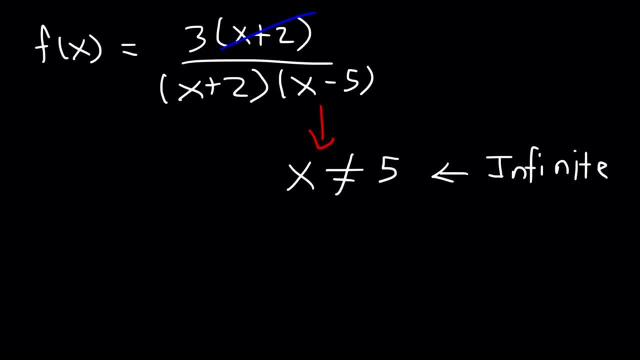 it's an infinite discontinuity. Now notice that we can cancel x plus 2.. However, this is still a point of discontinuity, So x cannot equal negative 2.. But this type of discontinuity is known as a whole, if it can be canceled. Here's another problem. f of x is equal to. 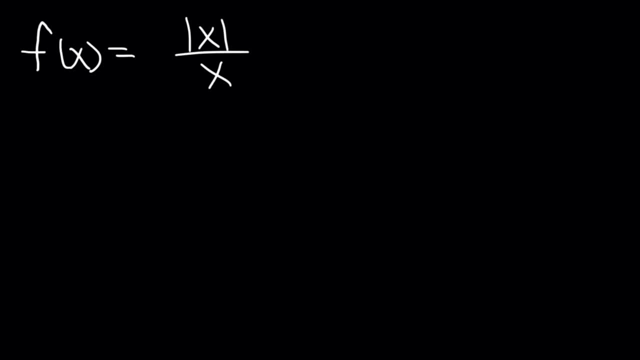 the absolute value of x divided by x. So what type of discontinuity do we have in this example? Is it a whole, a jump discontinuity or an infinite discontinuity? Also determine if it's removable or non-removable. Now we know that the denominator can be 0. So x cannot. 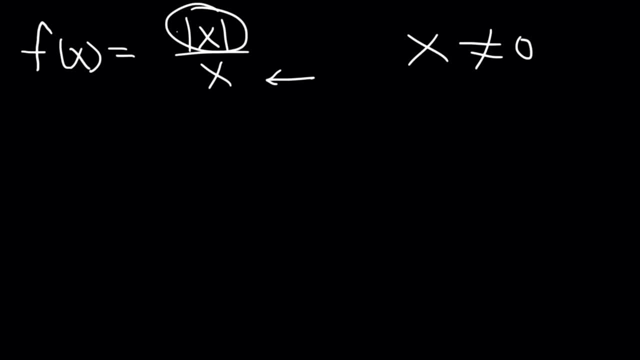 equal 0. But notice that we have an absolute value function. So this could be positive x, which means f of x can be 1, or it could be negative x, which means f of x can be equal to negative 1.. This is true when x is greater than 0, and this is true when x is less than 0. So 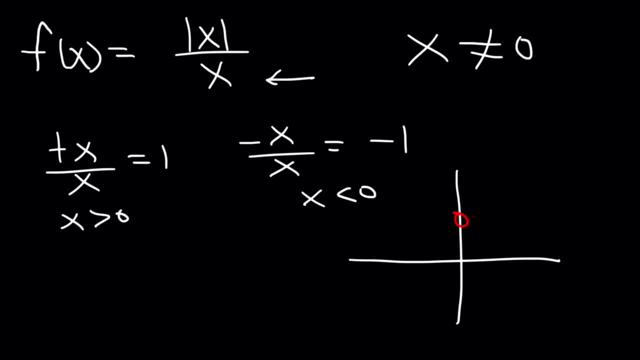 the graph looks something like this: When x is greater than 0,, it's going to be positive 1, and when it's less than 0, negative 1.. So this is the jump discontinuity, And it usually occurs whenever you have an absolute value function like this or it could. 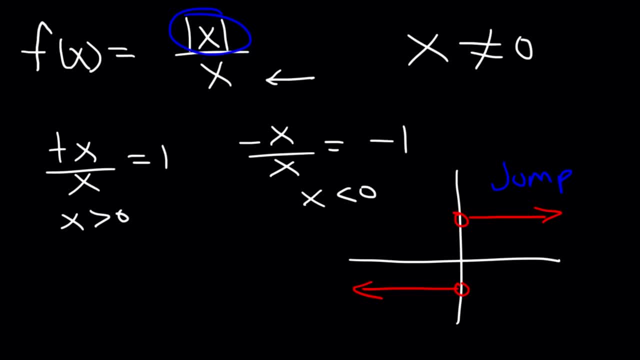 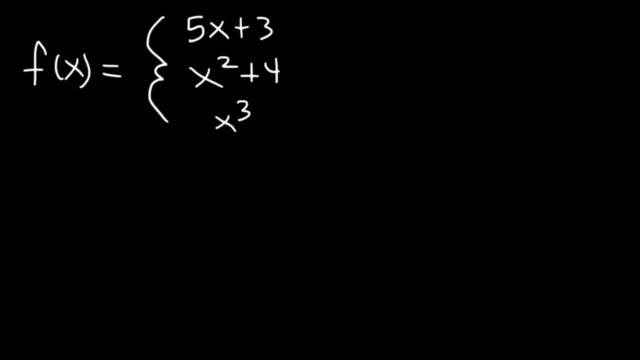 be due to a piecewise function as well. Now a jump discontinuity is also a non-removable discontinuity. The only one that's removable is the whole. Now let's say, if we have a piecewise function, 5x plus 3, x squared plus 4, and x cubed, So it's going to be 5x plus 3 when x is less. 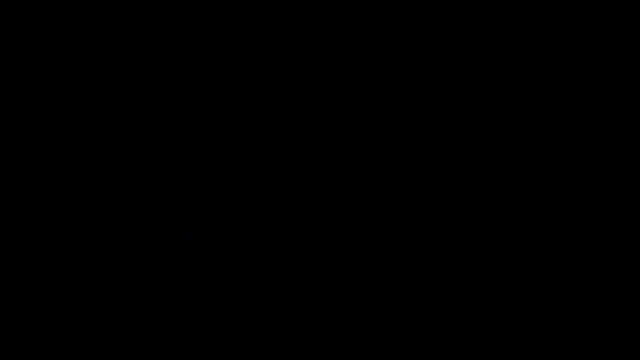 The only one that's removable is the whole. Now let's say, if we have a piecewise function, 5x plus 3, x squared plus 4. And x cubed, So it's going to be 5x plus 3 when x is less than 1.. 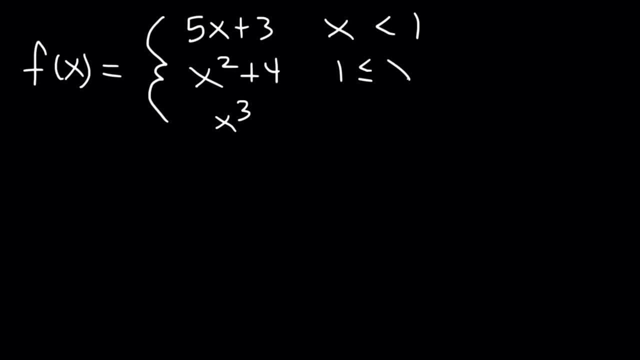 And when x is between 1 and 2. f of x is going to equal x squared plus 4.. And then it's going to be x cubed when x is equal to or greater than 2.. So determine the points of discontinuity. 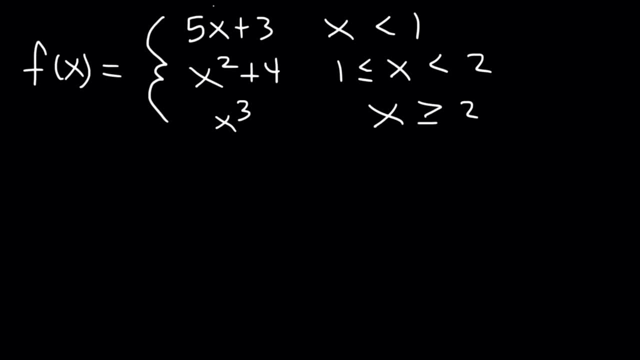 Now looking at this function. Linear functions are always continuous everywhere. Quadratic functions are also continuous, Even cubic functions. So any polynomial function is continuous everywhere. Rational functions like this one will be discontinuous when the denominator is 0.. 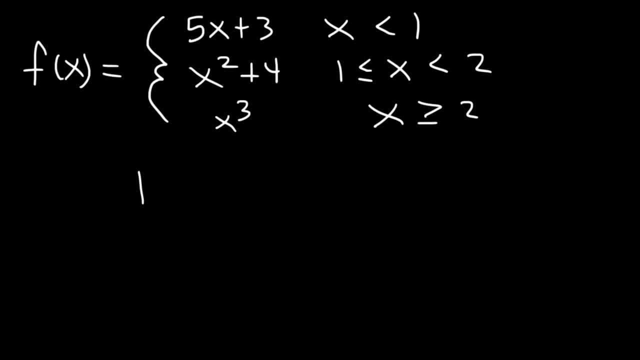 But we don't have a rational function here. So for a piecewise function the only possible locations where it can be discontinuous is at an x value of 1. Or at an x value of 2.. And a quick way to tell is to see if the y value is the same at those points. 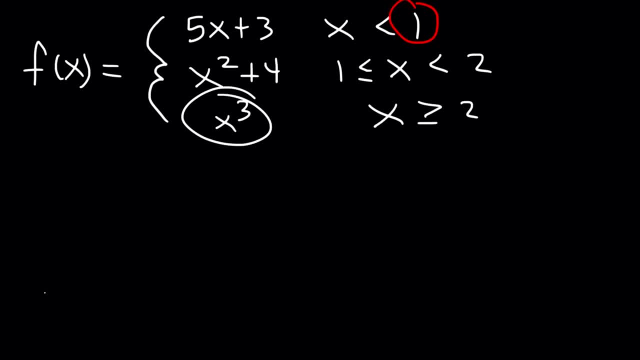 So let's start with 1.. If we plug in 1 into 5x plus 3., We're going to get a value of 8.. And if we plug it into the second part, x squared plus 4.- We're going to get a value of 5.. 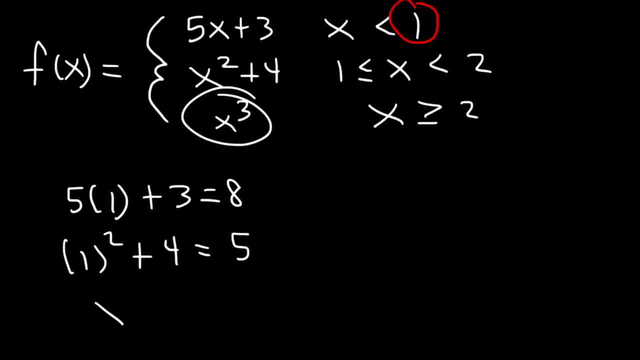 Therefore it's discontinuous at x equals 1.. Now what about at x equals 2?? So we need to use these two functions. If we plug in 2 into x squared plus 4. It's going to be 2 squared plus 4.. 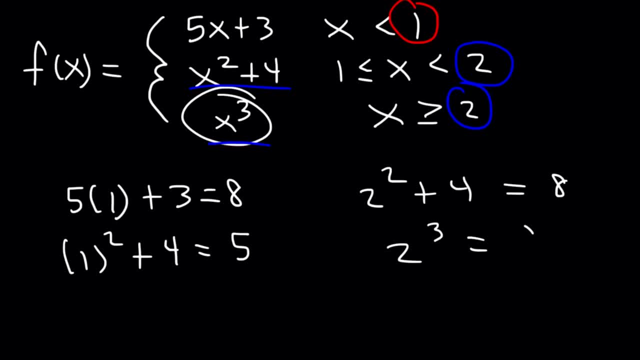 Which is 8.. And 2 to the third power is also 8.. Now, because these two have the same y value, You know that it's continuous at x equals 2.. So we're going to get a value of 8.. 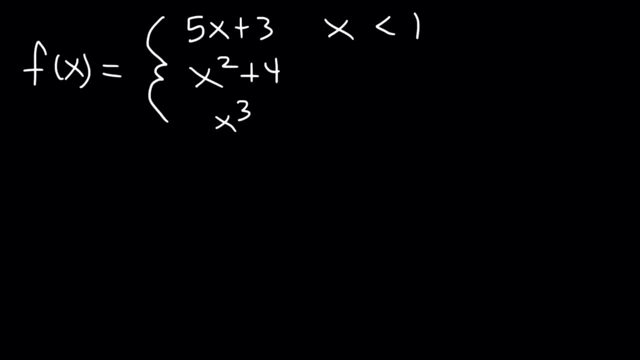 than 1, and when x is between 1 and 2, f of x is going to equal x squared plus 4.. And then it's going to be x cubed when x is equal to or greater than 2.. So determine the points of discontinuity. 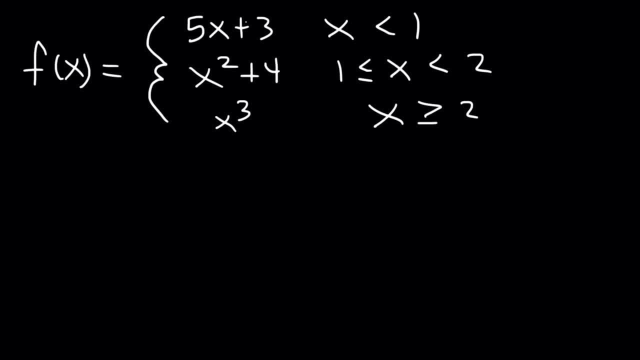 Now looking at this function. linear functions are always continuous everywhere. Quadratic functions are also continuous, even cubic functions. So any polynomial function is continuous everywhere. Rational functions like this one will be discontinuous when the denominator is 0. But we don't have a rational function here. So for a piecewise function, the only. 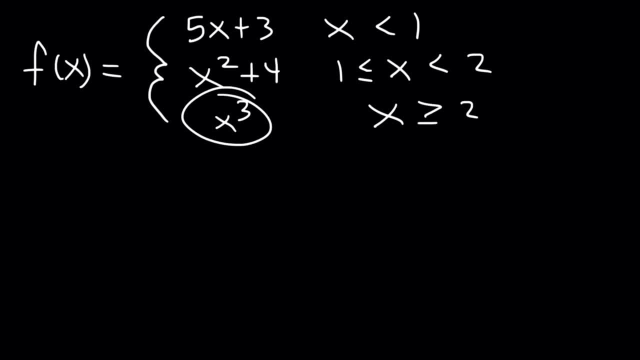 possible locations are the points of discontinuity. Where it can be discontinuous is at an x value of 1 or at an x value of 2.. And a quick way to tell is to see if the y value is the same at those points. 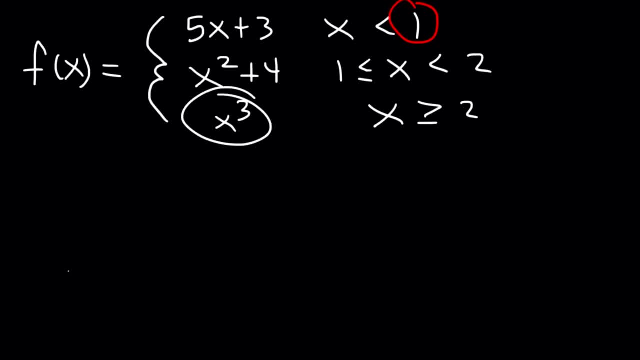 So let's start with 1.. If we plug in 1 into 5x plus 3, we're going to get a value of 8.. And if we plug it into the second part, x squared plus 4, we're going to get a value. 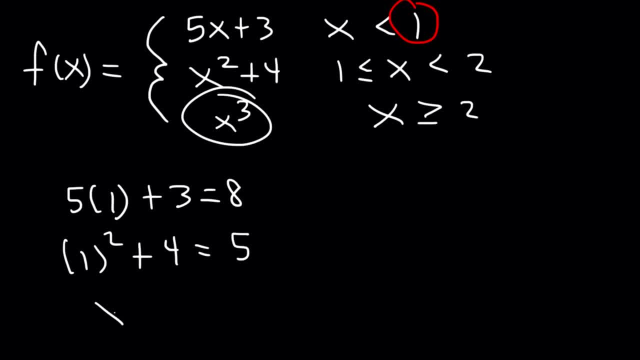 of 5.. Therefore it's discontinuous. at x equals 1.. Now what about at x equals 2?? So we need to use these two functions. If we plug in 2 into x squared plus 4, it's going to be 2 squared plus 4, which is 8.. 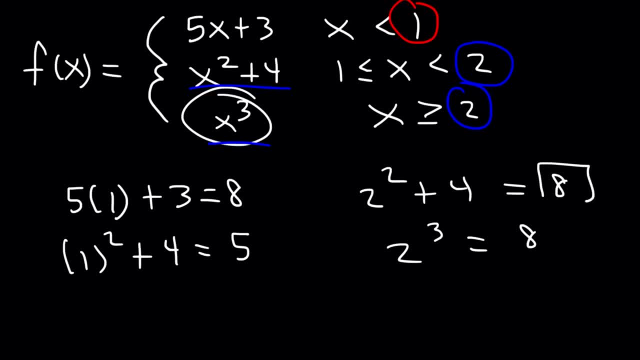 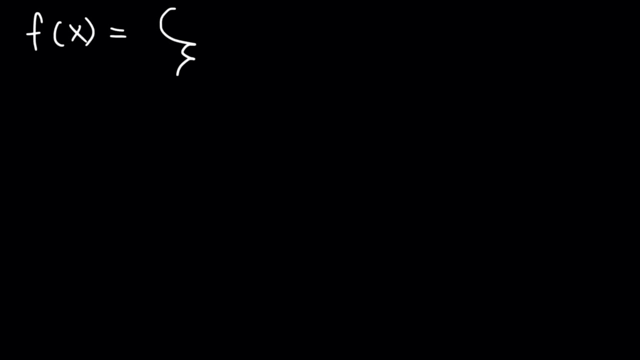 And 2 to the third, power is also 8.. Now, because these two have the same y value, you know that it's continuous at x equals 2.. But it's discontinuous at x equals 1.. Consider the function f of x, which is equal to cx. 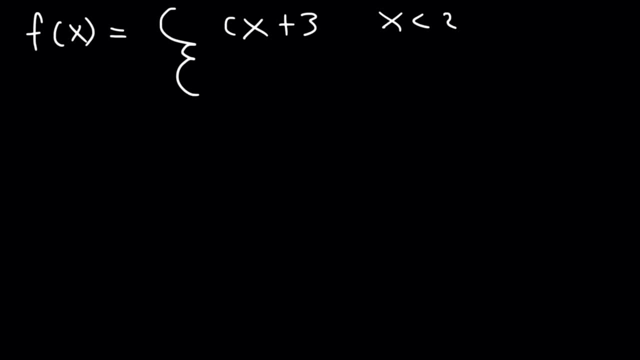 cx plus 3 when x is less than 2.. And that's equal to 3x plus c when x is equal to or greater than 2.. What is the value of the constant c that will make the function continuous at x equals 2?? 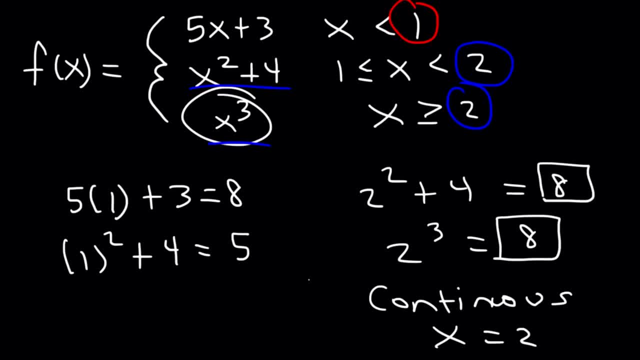 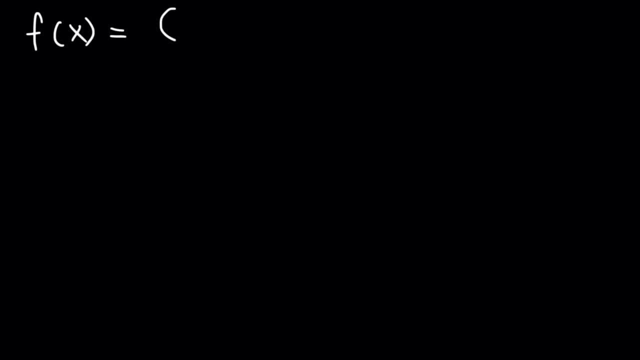 But it's discontinuous. at x equals 1. Consider the function f of x, Which is equal to cx plus 3.. When x is less than 2. And that's equal to 3x plus c. When x is equal to. 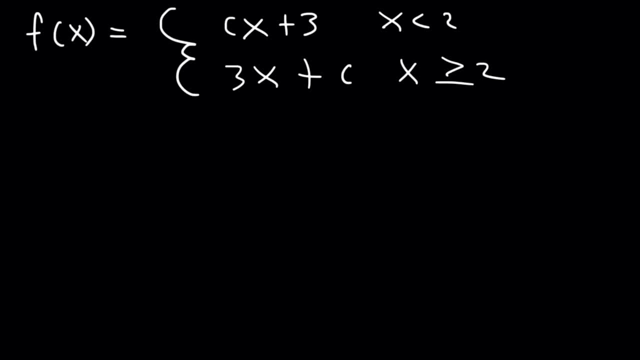 Or greater than 2.. When x is greater than 2. Or greater than 0. What is the value of the constant C that will make the function continuous at x equals 2?? So what do we need to do in order to find the value of that constant C? 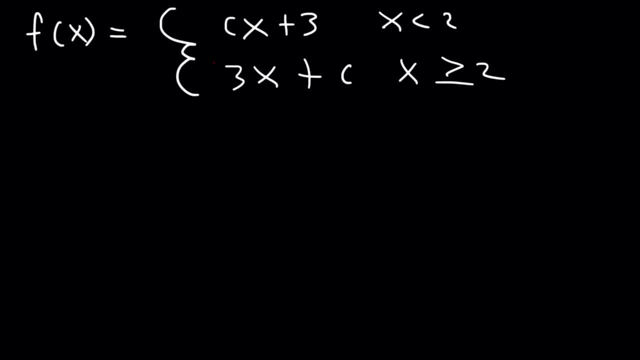 Well, if it's going to be continuous, at x equals 2,, these two functions have to have the same y value, which means that they must be equal to each other. So the first thing is to set them equal to each other, and they have to be equal to each. 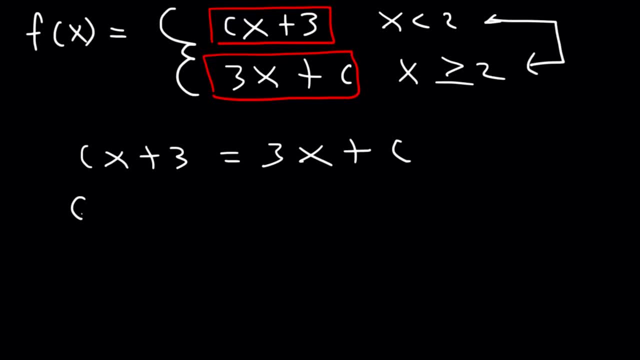 other at an x value of 2.. So the second step is to replace x with 2, and then find the value of C. So we're going to have: 2C plus 3 is equal to 6 plus C. So let's subtract both sides by C and let's subtract both sides by 3.. 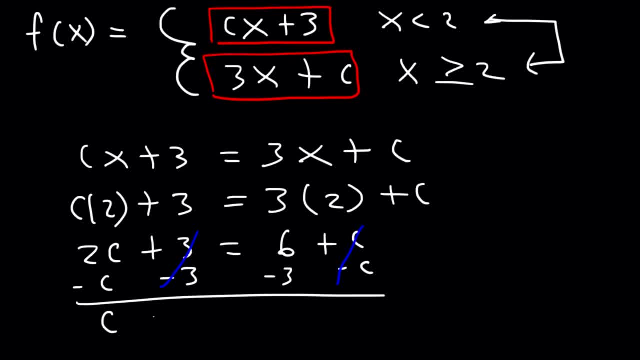 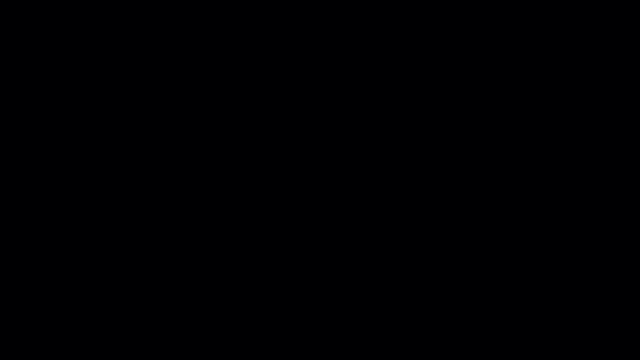 2C minus C is C, 6 minus 3 is C, 3 is 3.. So C is equal to 3.. Now, what about this problem? Let's say that f of x is equal to ax minus 2, and also x squared minus 5, when x is less. 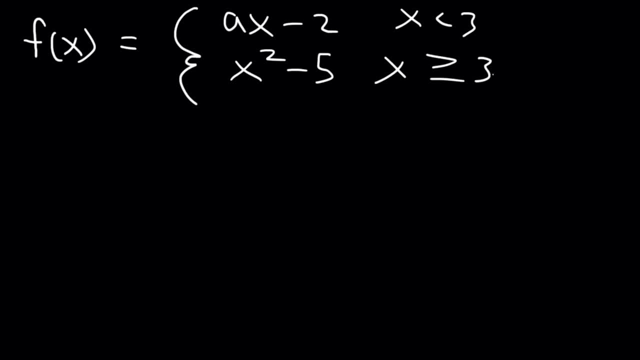 than 3, and when x is equal to a greater than 3.. Find the value of the constant A. That will make the function continuous. So go ahead, pause the video and try this problem. The first thing we need to do is set the two portions of the function equal to each other. 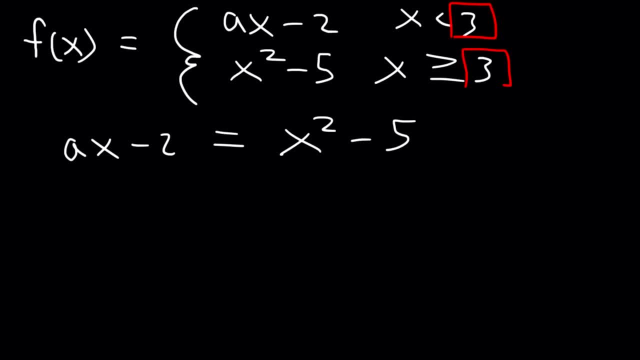 and then in the next step, we need to replace x with 3.. So this is going to be: A times 3 minus 2 is equal to 3 squared minus 5.. 3A minus 2 is equal to 9.2.. 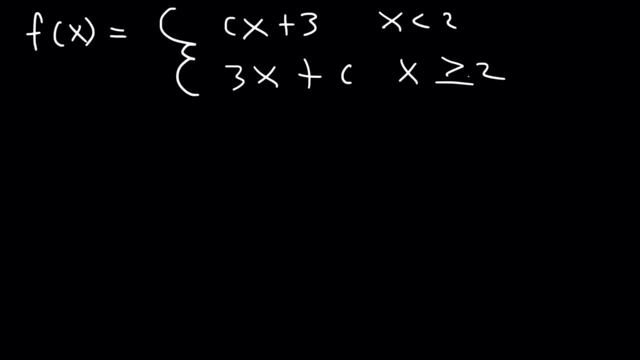 So what do we need to do in order to find the value of that constant c? Well, if it's going to be continuous- at x equals 2,, then we need to find the value of the constant c. These two functions have to have the same y value, which means that they must be equal to each other. 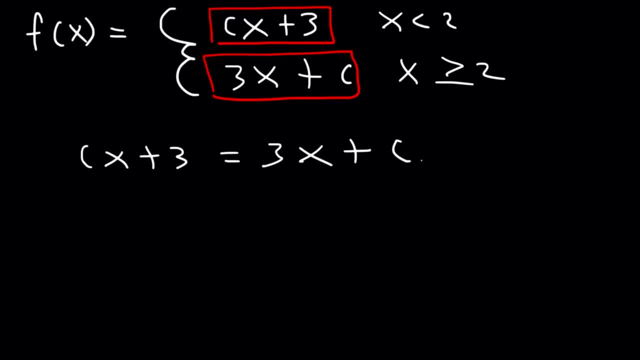 So the first thing is to set them equal to each other, And they have to be equal to each other at an x value of 2.. So the second step is to replace x with 2 and then find the value of c. 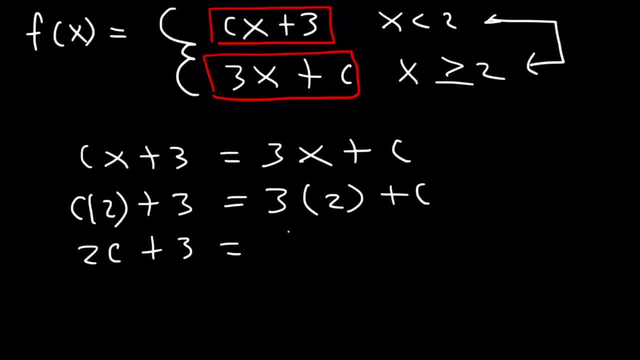 So we're going to have: 2c plus 3 is equal to 6 plus c. So let's subtract both sides by c and let's subtract both sides by 3.. So we're going to have 2c minus c is c. 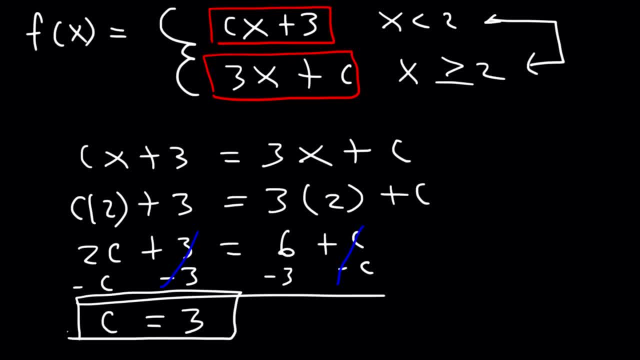 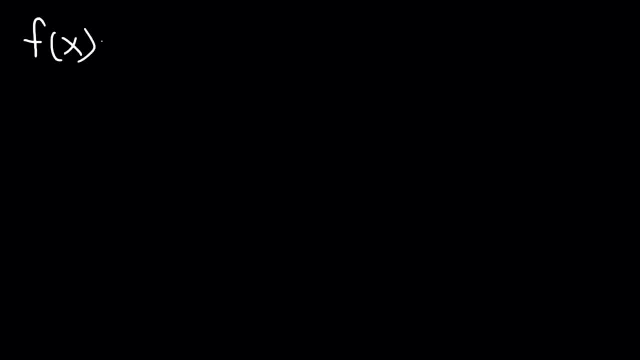 6 minus 3 is 3.. So c is equal to 3.. Now, what about this problem? Let's say that f of x is equal to ax minus 2, and also x squared minus 5.. When x is less than 2, we're going to have x squared minus 5.. 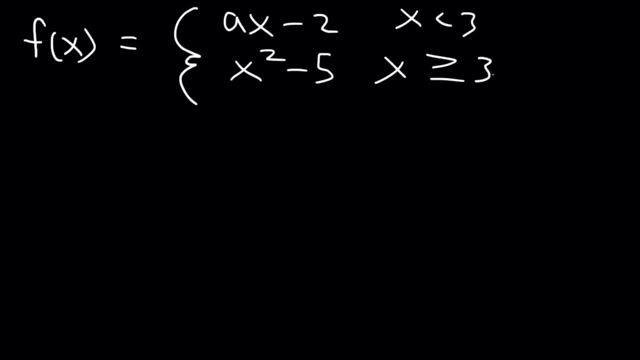 When x is less than 3 and when x is equal to or greater than 3.. Find the value of the constant a. that will make the function continuous. So go ahead and pause the video and try this problem. So the first thing we need to do is set the two portions of the function equal to each other. 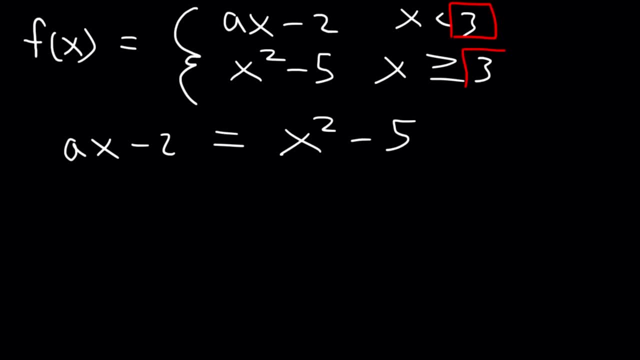 And then in the next step, we need to replace x with 3.. So this is going to be: a times 3 minus 2 is equal to 3.. So this is going to be 3a minus 2, which is equal to 9 minus 5.. 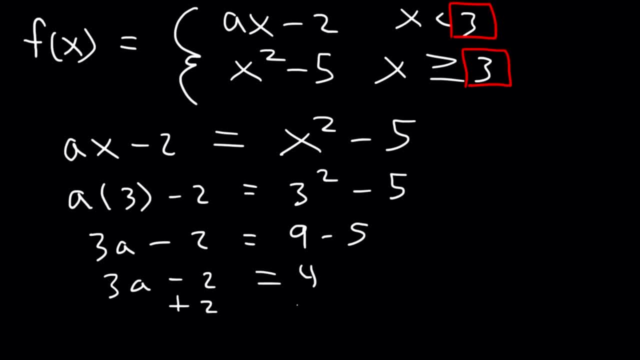 And 9 minus 5 is 4.. Now if we add 2 to both sides, 4 plus 2 is 6.. And then we have to divide both sides by 3.. So 6 divided by 3 is 2.. 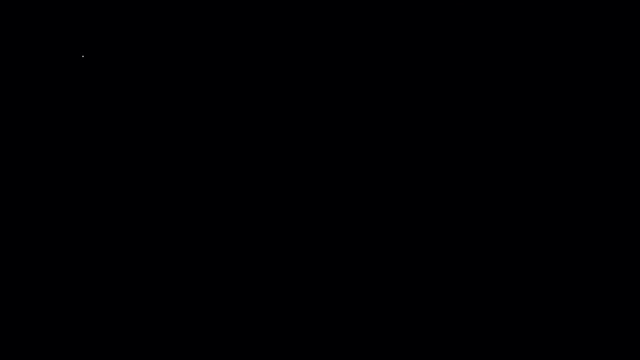 So the value of the constant is 2.. Let's try another problem. So let's say f of x is ax plus 5, when x is less than 1. And that it's x squared minus bx plus 9, when x is between 1 and 4.. 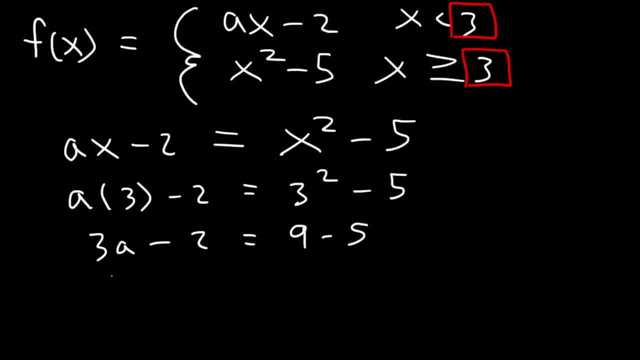 1 minus 2 is equal to 9.2.. Let's see how that works. Here's our problem: 9 minus 5.. And 9 minus 5 is 4.. Now, if we add 2 to both sides, 4 plus 2 is 6.. And then we. 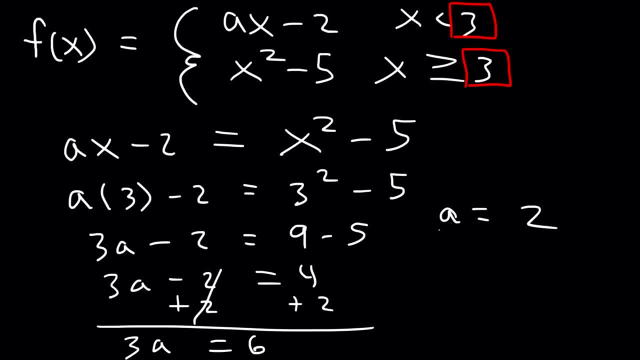 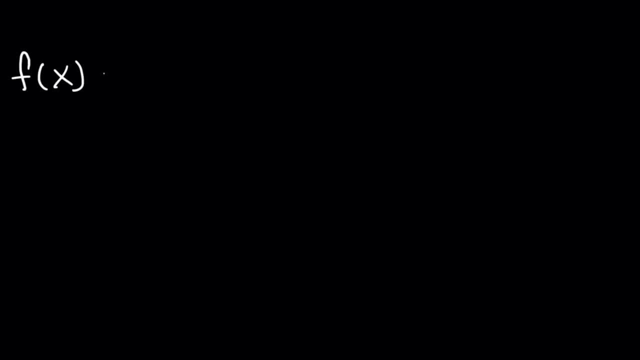 have to divide both sides by 3.. So 6 divided by 3 is 2.. So the value of the constant is 2.. Let's try another problem. So let's say f of x is ax plus 5 when x is less than 1.. 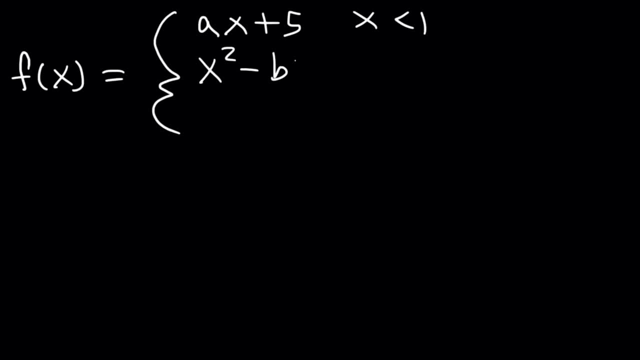 And that it's x squared minus bx plus 9 when x is between 1 and 4.. And it's ax squared minus bx minus 7 when x is equal to or greater than 4.. Go ahead and find the values of a and b. So first let's make the function continuous when x is 1.. So therefore we need to set. 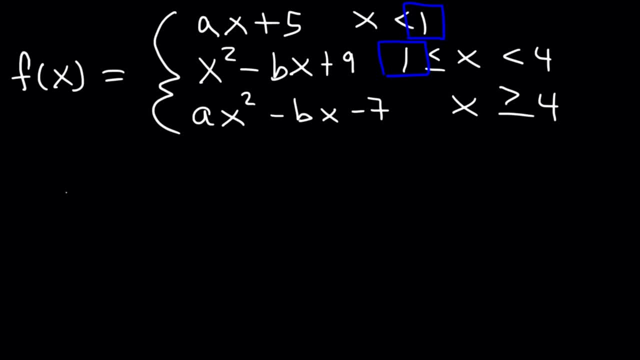 these two equal. So ax plus 5 is equal to x squared minus bx plus 9.. Now let's replace x with 1.. So this is going to be 1a or just a. 1 squared is 1 minus b times 1, or b plus 9.. 1 plus 9. 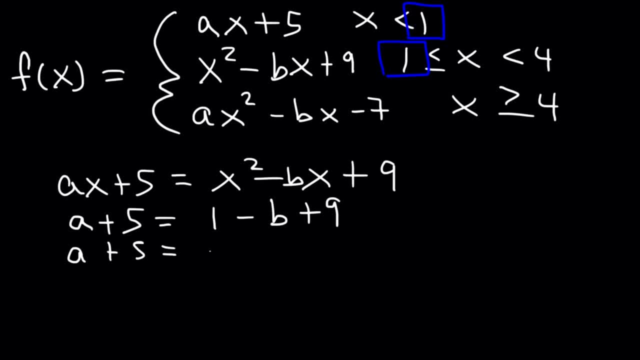 is 10.. So a plus 5 is equal to 10 minus b. Now let's add b to our equation, So we have 3 squared minus b, squared plus 9.. y squared minus 5 is equal to 5. And the other way. 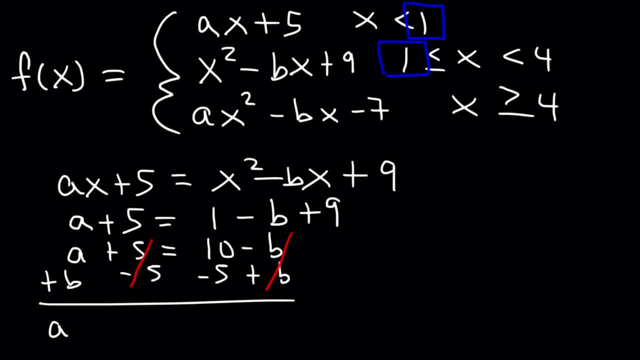 around. Let's subtract both sides, So a plus b is equal to 5.. So on the left, what we have is a plus b. On the right, we have 10 minus 5.. So a plus b is equal to 5.. Now let's use: 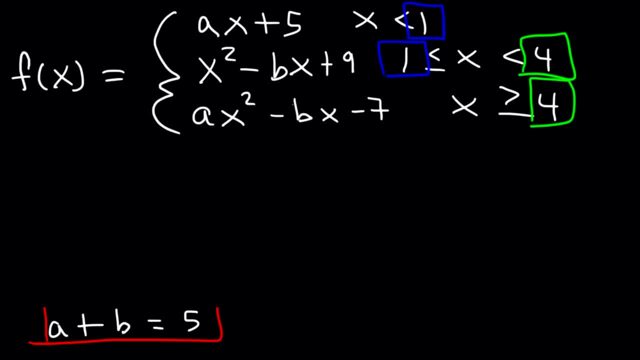 the next number: 4. 4. 0.. 4. 0.. 0. 0.. We need to set these two functions equal to each other. So x squared minus bx plus 9 is equal to ax squared minus bx minus 7.. 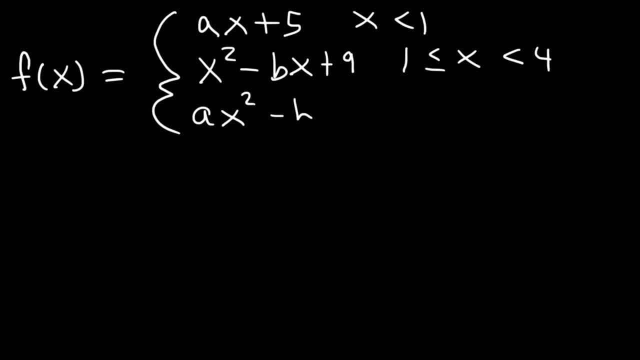 And it's ax squared minus bx minus 7, when x is equal to or greater than 4.. Go ahead and find the values of a and b So first. So let's make the function continuous when x is 1.. 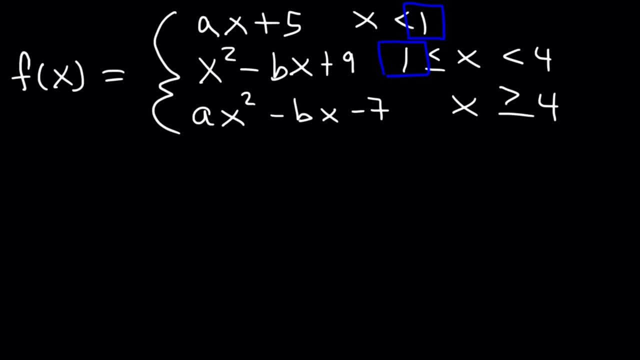 So, therefore, we need to set these two equations equal to each other. So ax plus 5 is equal to x squared minus bx plus 9.. Now let's replace x with 1.. So this is going to be 1a, or just a. 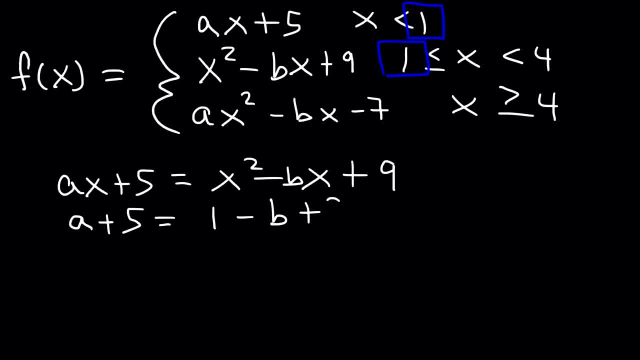 1 squared is 1 minus b times 1, or b plus 9.. 1 plus 9 is 10.. So a plus 5 is equal to 10 minus b. Now let's add b to both sides And let's subtract both sides by 5.. 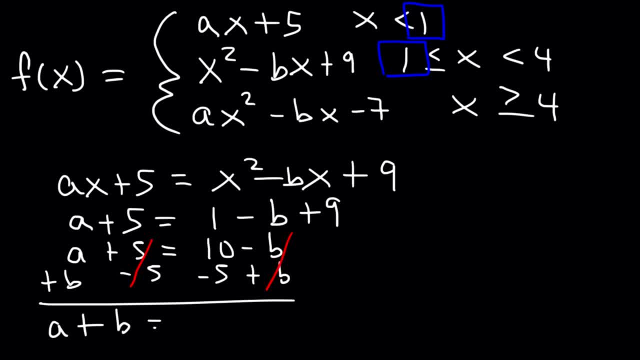 So on the left, what we have is a plus b. On the right, we have 10 minus 5.. So a plus b is equal to 5.. Now let's use the next number, 4.. So we need to set these two functions equal to each other. 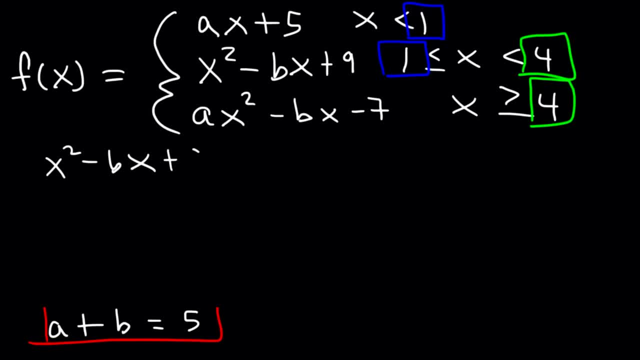 So x squared minus bx plus 9 is equal to ax squared minus bx minus 7.. And x is 4.. So 4 squared minus 4b plus 9 is equal to 4 or a times 4 squared. So x squared minus 4b plus 9 is equal to 4 squared minus b times 4 minus 7.. 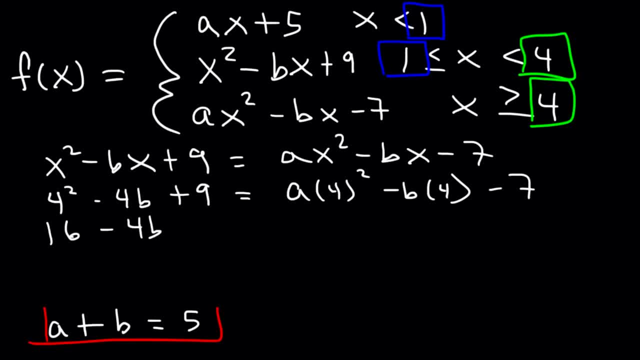 So 4 squared is 16. And this is going to be 16a minus 4b minus 7.. So if we add 4b to both sides, notice that we can cancel the b expressions, since they're the same. 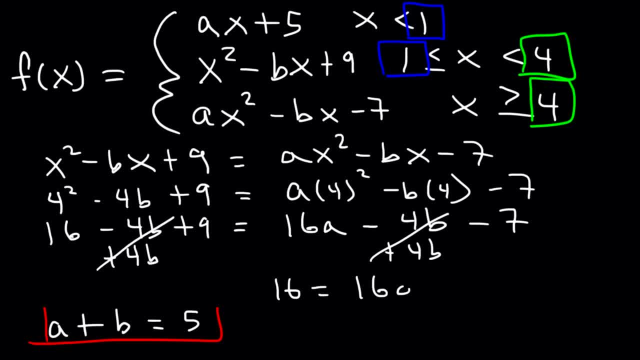 So, therefore, 16 is equal to 16a minus 7.. And let's not forget about the plus 9 on that side. 16 plus 9 is 25. And that's equal to 16a minus 7..